0.. 2s is equal to 0. 2bc equals 0.. 2a equals 0.. 2bc equals 0. 2bc equals 1. 2bc equals 1. 2bc equals. 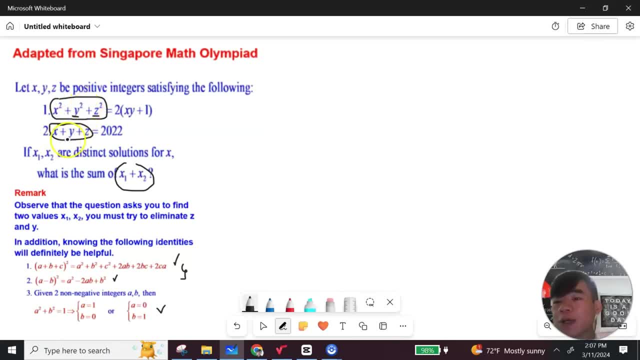 have SYZ. Alright, we try to eliminate this one. so I try to make the second one square. okay? So I have S plus Y plus Z- equal 2022, right, So I square both sides so it turns out to be S plus Y plus Z, square right, Equal 2022.. Alright, now I expand this one using: 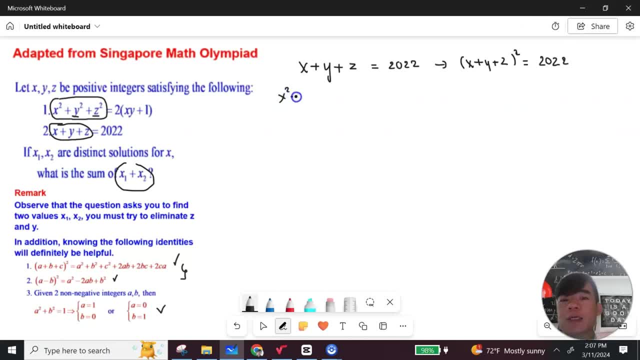 the formula right here. So it turns out to be S square plus Y square plus Z square plus 2SY plus Z square, 2YZ plus 2SZ equal 20,, oh sorry, 22 square. Alright, I'm gonna use the information, right. 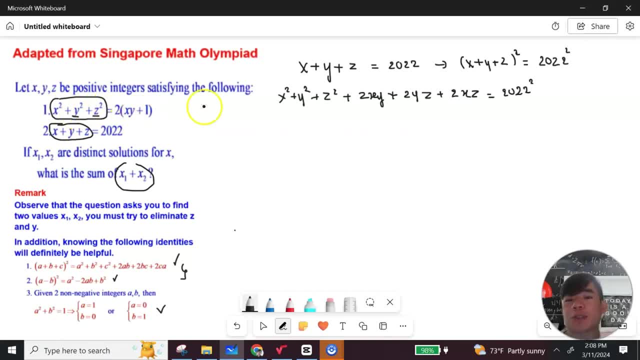 here S square plus Y square plus Z square, equal this one. so I just replace this guy right here with this guy, okay, So I have what? 2SY plus 2, right, I distribute this one. Equal 2SY plus 2YZ plus 2SZ, equal 2022 square. 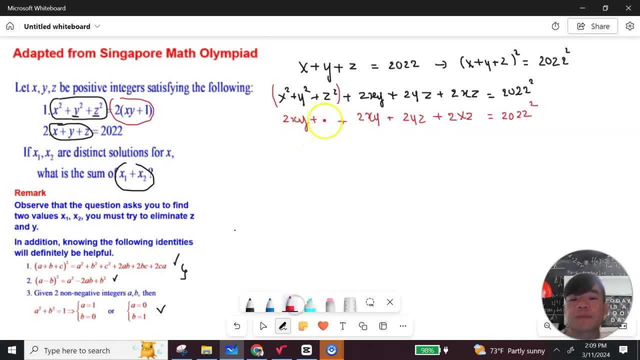 Alright, Alright. so next, 2SY plus 2SY is equal to 4SY right, 4SY Alright plus plus 2.. Now this one: I have Z right. This is a common factor. I factor 2Z out, so it's gonna be 2022. 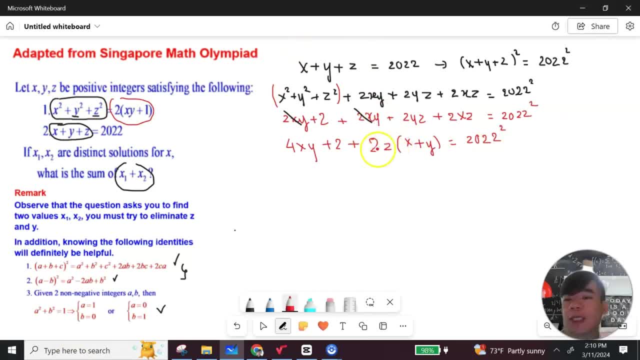 square. okay, Z right here. Z can be equal to what Z right here. Equal 2022 minus S plus Y. right, So I have 4SY plus 2 plus 2 times 2022 minus S plus Y. Alright. 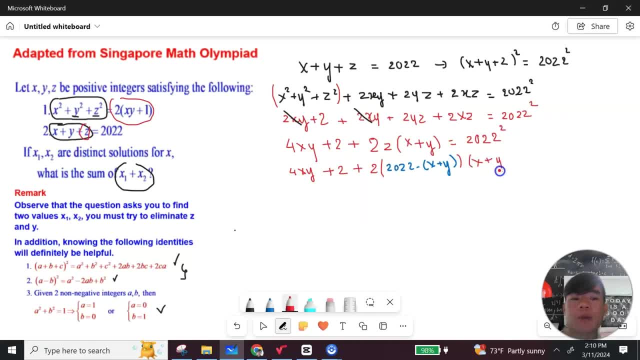 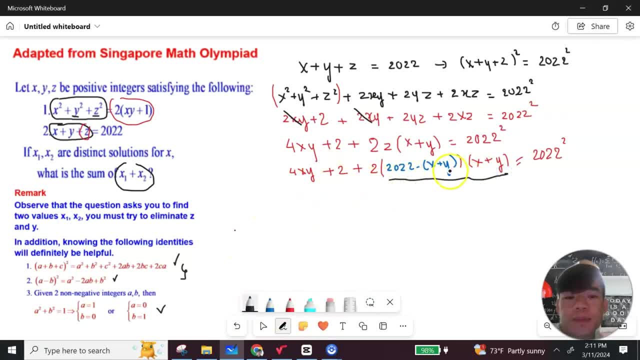 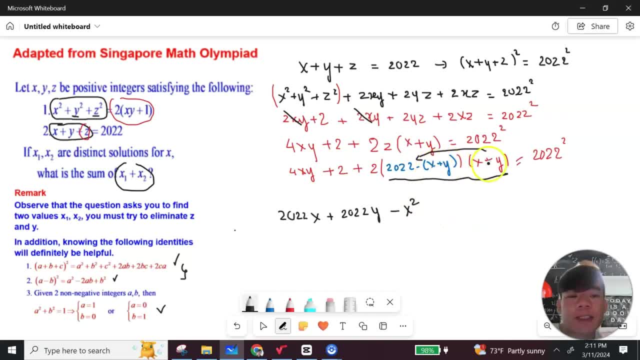 going to be x squared and I have a negative sign. so negative: x squared, x times y. okay, and then x times y is x squared. y times x is going to be x squared. so 2x squared and negative: right. so it's going to be negative: 2x squared. and then last one: y times y is. 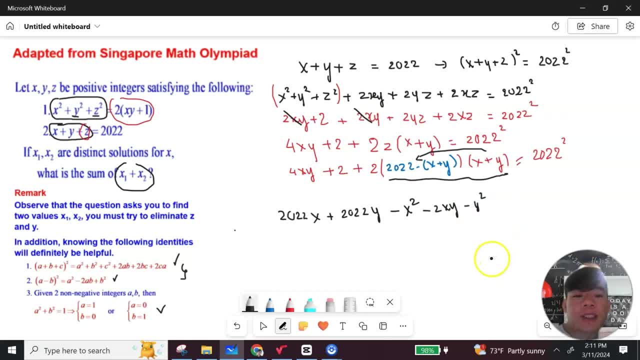 going to be y squared, so it's going to be negative y squared, all right. so I just rewrite: so this one is going to be what? 4xy plus 2,, all right, plus 2 times 20,, 20,, 2s plus. 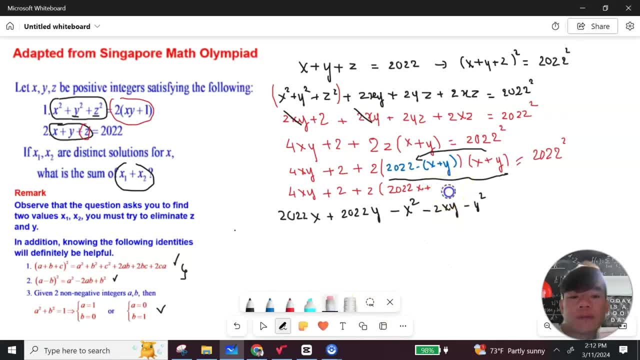 20,, 20,, 2.. 20,, 20,, 2, y minus x squared minus 2xy minus y squared, equal 20, 20, 2 squared. okay, 4xy right here, plus 2,. now I distribute this, so it could be 4,, 40,, 44, x. 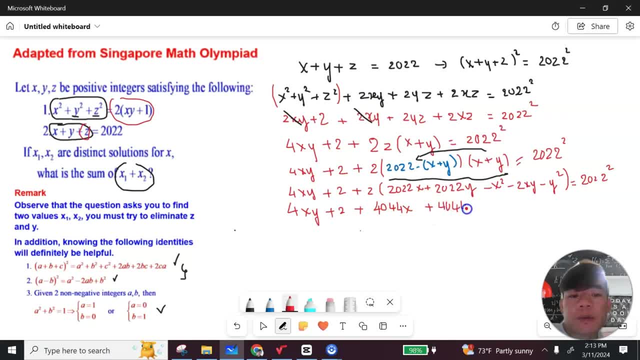 plus 40,, 44, y minus 2x squared minus 4xy. all, right now I simplify: 4x squared right here and negative 4x squared right here, gone, okay. so I'm going to end up with what negative. 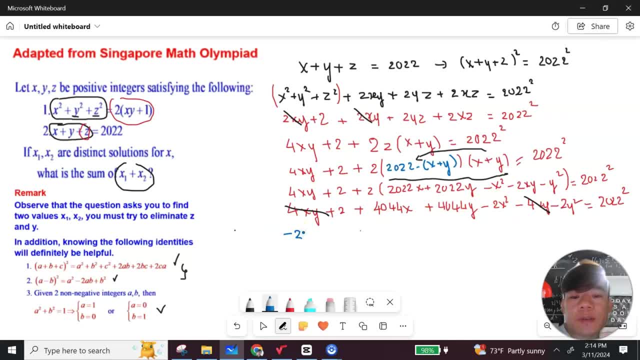 2x squared right here, All right. plus 40, 44x. then minus 2y squared plus 40, 44y plus 2, equal 20,, 20, 2 squared, all right. now I subtract negative 20, 22 square both sides and subtract 2 both sides. 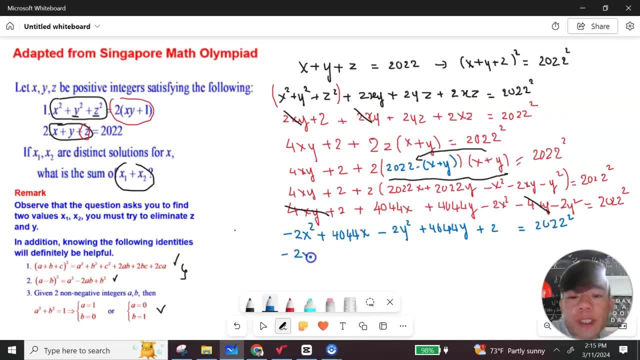 okay. so I'm going to end up with negative 2x squared minus ah plus 40, 44x. minus 2y squared plus 40, 44y. All right, All right. minus 20, 22 squared, equal negative 2,. okay, and I multiply both sides by negative. 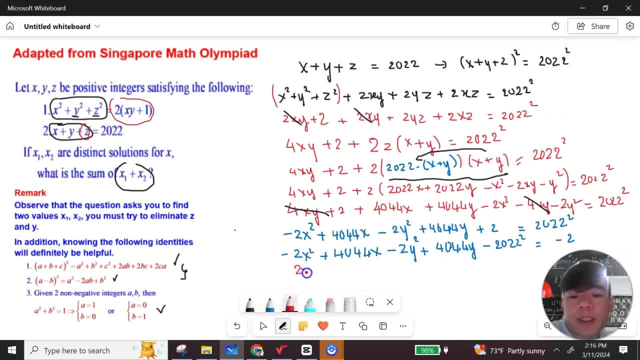 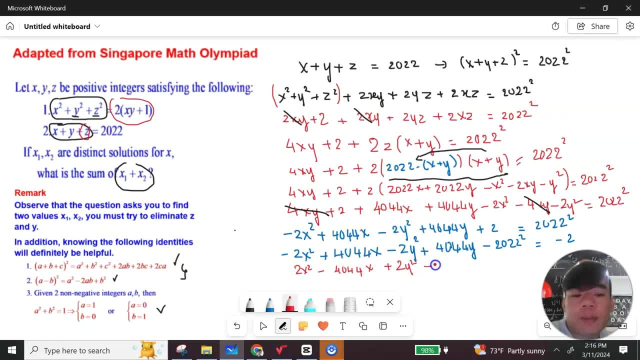 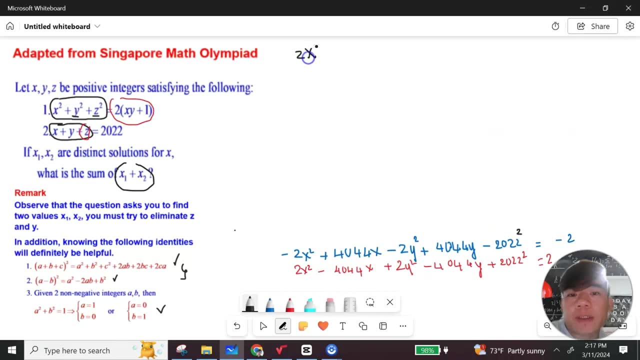 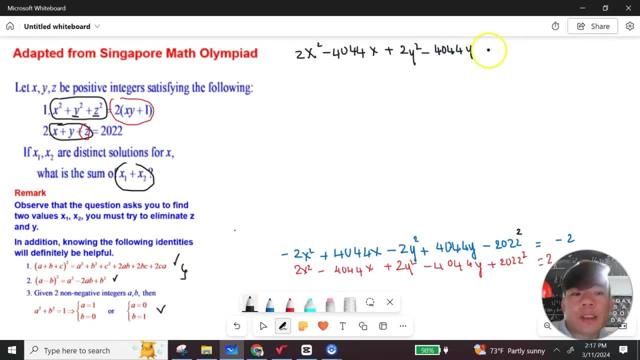 All right, All right, y plus 20, 22. square equal to: okay, now, right here. okay for this, this one. i wrote: this guy, this guy, this guy and this guy right here, okay, so i factor two out, so i have two. let's give me s square minus 20, 22 s. all right, plus 2. y. square minus 20, 22 y. 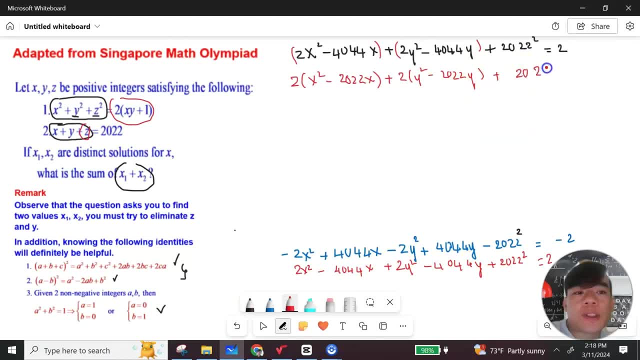 plus 20, 20 to square, equal to okay. next one: i, this one i need to do come this square, okay. so i'd realize two right here. this is the first one, right. this is the second one right here. this is the third one, right? this is the third one, right. this is the fifth one right and this is the third one. 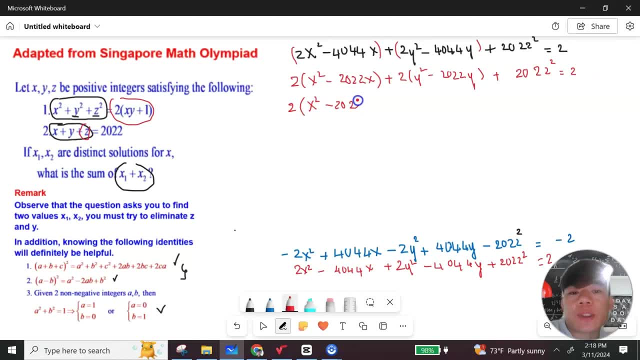 to x: square right here minus 20, 22x- okay. plus alright, blank okay. plus 2y square here, minus 20, 22y, plus blank right here, okay, and then plus 20, 22 square equal 2,. 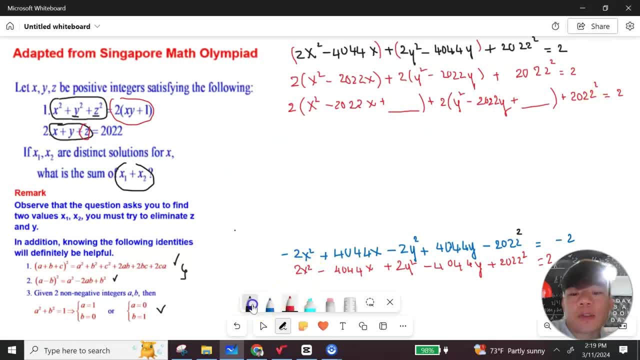 okay, alright. so you need to fill in the blank right here in order to make it 1: commit, square. alright. take the middle term right here: divide by 2 and square, so it's 20,, 22,. divide by 2,, it could be 10.. 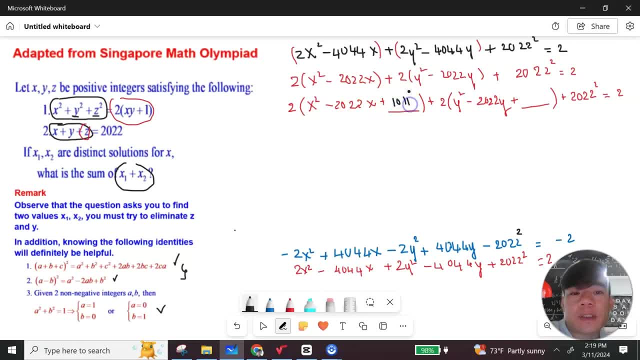 11 and square should be 10, 11 square, and this is same thing: 10, 11 square. now you just literally add 10, 11 square, right? and then, don't forget, multiply by 2,, so basically: 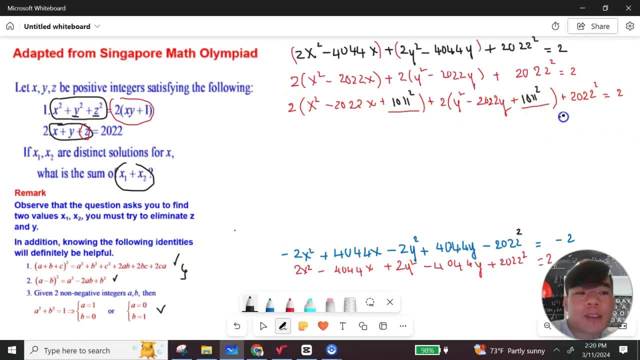 right here. you just add this and you need to subtract. right, you need to subtract 2 times this one and this is 2 times this one. so it should be 4 times 10, 11 square and this is 4 times 10, 11 square. alright, the first 3 right here becomes a complete square. 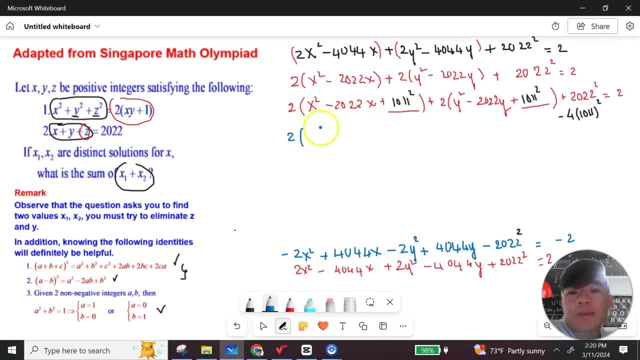 so you have what: 2 times x minus 10, 11 square- alright, plus 2y minus 10, 11 square- alright, equal this guy. and this guy actually cancel out y okay, because you now have x minus. 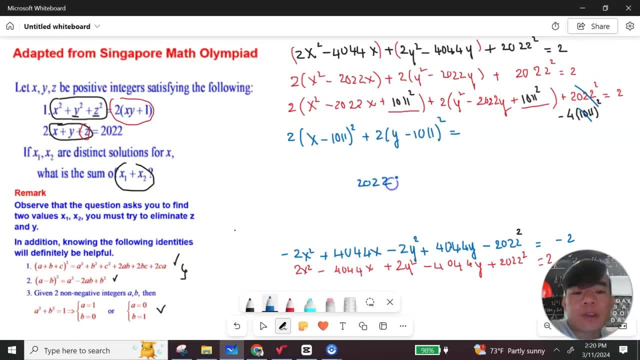 10, 11 square. so you now look 20, 22 square. can I rewrite this one as 2 times 10, 11 all together square? alright, so then I just write this one: 2 square times 10, 11, square 2. 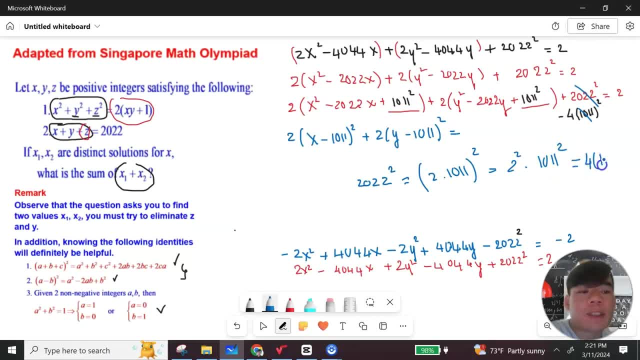 square, it could be 4, so it could be 4 times 10, 11 square. you see that, and this is exactly this one. This one is gone, so the answer should be 2, on the right-hand side only, alright, next. 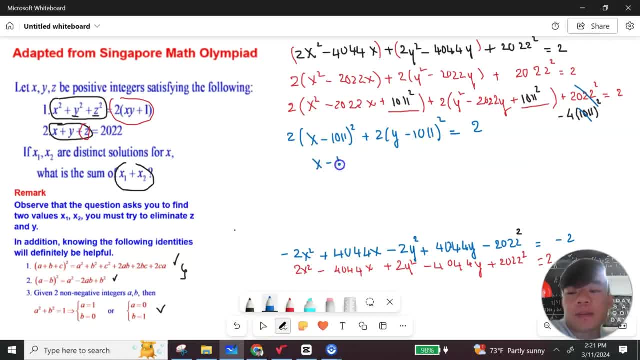 one add the variables up by 2, so I have what x minus 10, 11 all together, square, plus y minus 10, 11 all together, square, equal 1,. alright, so since x and y are integers, 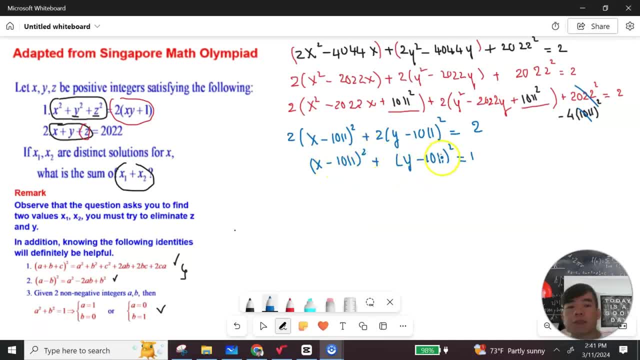 then x minus 10, 11 square plus y minus 10, 11 square equal 1, either one of these should be 1 or 0,. okay, so I have the first case: x minus 10, 11 equal 1, y minus 10, 11 equal. 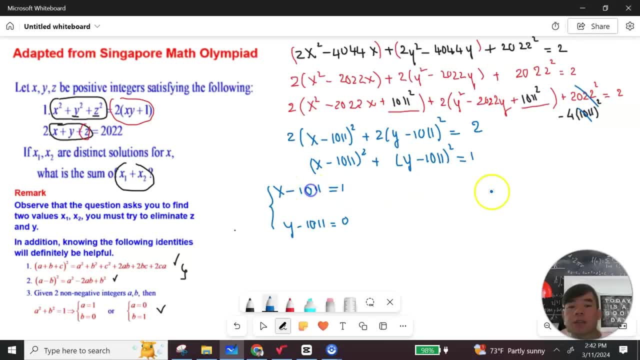 0.. The second case: x minus 10, 11 all together square 1.. What minus 10, 11 equals 0.. y minus 10, 11 equals 1.. So solve the first case s equals 10, 12.. y equals 10, 11..